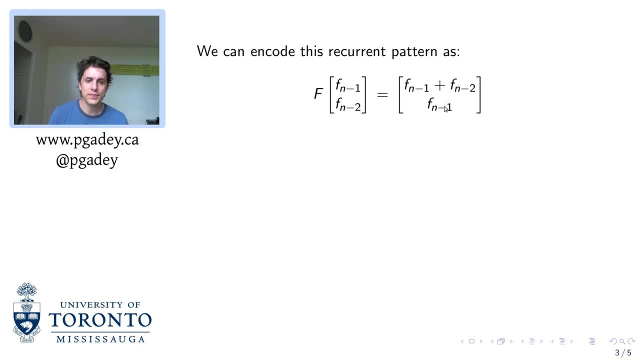 going to be fn, fn-1.. So we take fn-1, fn-2, add them together to give us fn. If we want to take this right hand side and write it in a more linear algebra way, we can write it as: 1 times fn minus 1 plus 1 times fn minus 2.. 1 times fn minus 1 plus 0 fn minus 2.. 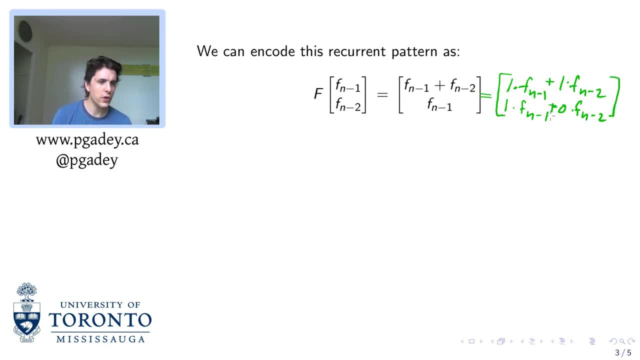 This is going to be fn- fn minus 1 plus 1 plus 2, fn minus 2.. Okay, so this is starting to look more and more like a matrix, and we can get a value for this matrix f in the following way: We extract out the coefficients of that matrix and we get the. 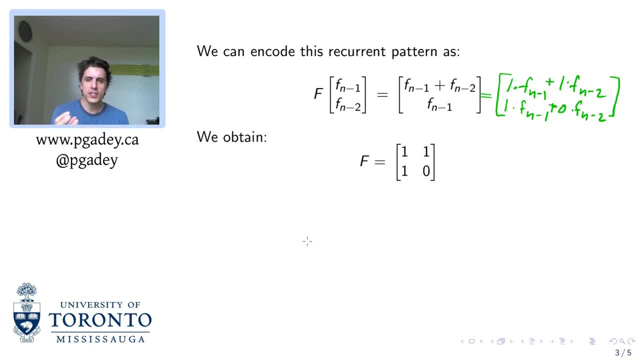 matrix 1110.. So this matrix encodes the process of calculating the Fibonacci numbers for us. How can we use it? We'll multiply it by the first two Fibonacci numbers. This is going to be fn. fn minus 1 plus 1.. 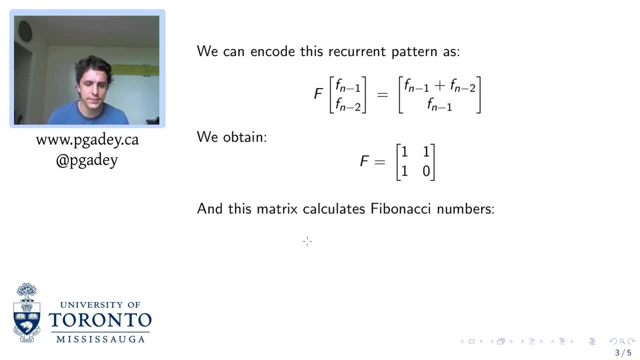 This is going to be fn. fn minus 1 plus 2, fn minus 5.. This is going to be fn. fn minus 1 plus 1 plus 2.. Fibonacci numbers. and see what we get. When we multiply this by 1, 1, we get 2, 1,. the next pair. 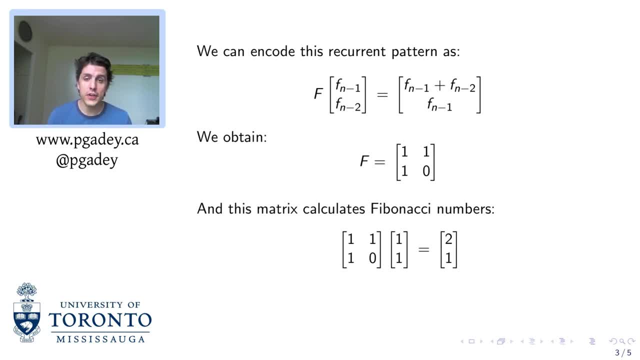 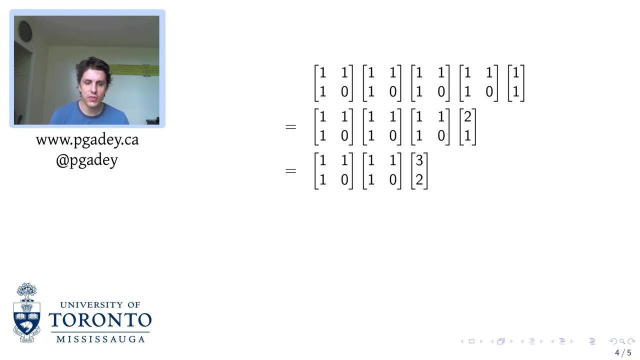 of Fibonacci numbers Not super duper impressive, but let's try it with a higher power. Okay, now, when we've got four of these matrices, watch what happens. The first multiplication gives us 2, 1.. The next multiplication gives us 3,, 2.. The next 5,, 3.. The next 8, 5.. Every time we do a matrix, 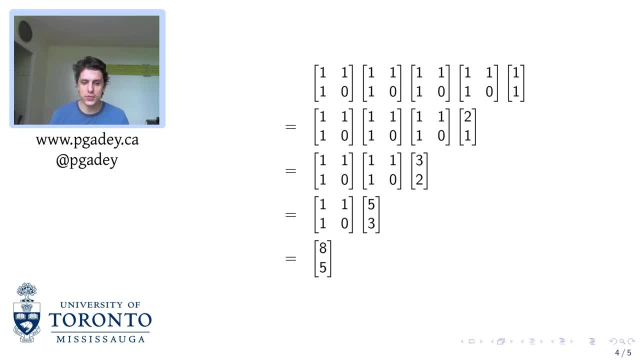 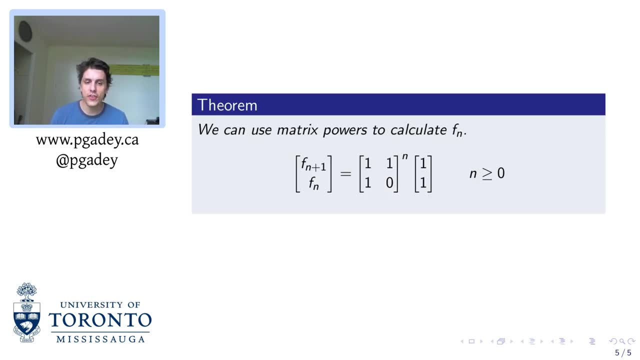 multiplication, we get the next pair of Fibonacci numbers. So let's make this into a theorem. We can use matrix powers to calculate the Fibonacci numbers fn. The formula to do so is given in this theorem. I think this is a really interesting application of linear algebra. 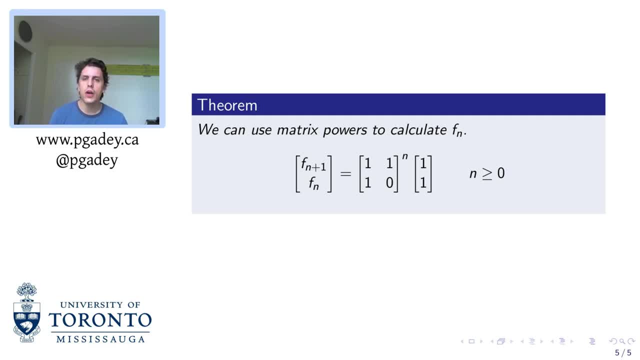 because it shows us how to calculate the Fibonacci numbers. fn. We can use linear algebra to model recursive processes and calculate these seemingly ubiquitous numbers, the Fibonacci numbers. Thanks for watching.